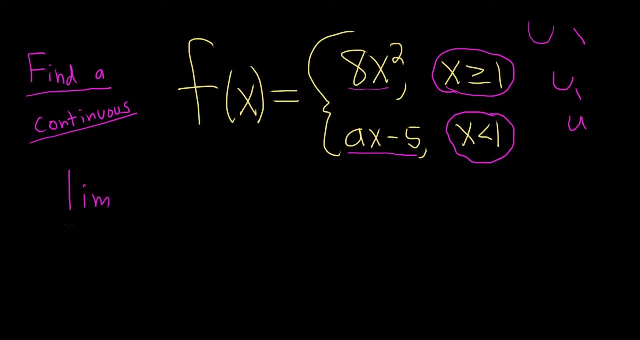 force the limit to exist. Let's start by taking the limit from the left. So if we take the limit from the left, we're going to use the bottom piece, because that means x is less than one. So I'll go ahead and put the f of x here. And so, because we're approaching from 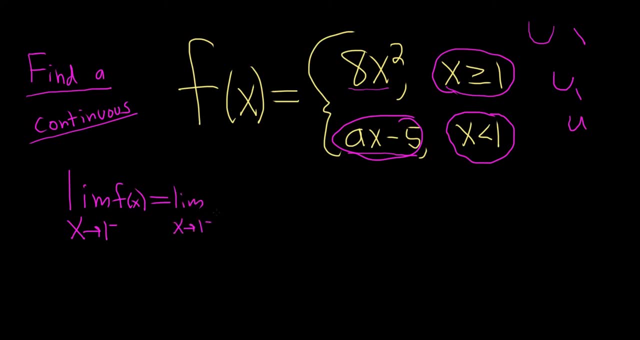 the left. just to show an extra step, we replace f of x with ax minus five right, Because from the left x is less than one. And if you don't see that, just draw a picture. Here's one. Here's x, because you're approaching from the left. Oh yeah, it's a smaller number. 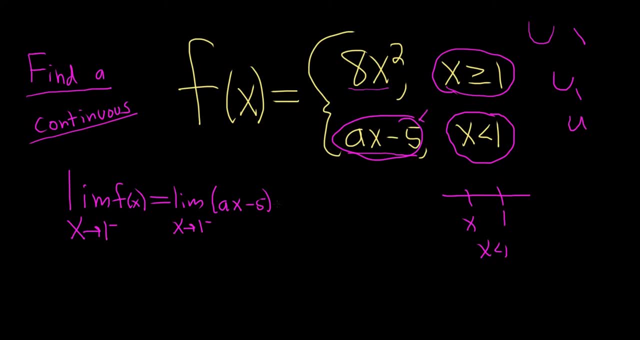 X is less than one, So we use this piece. Now we can go ahead and plug in the one. When we do that, we drop the limit sign, So it's a times one, which is just a minus five. Now let's take the limit from the left, So we're going to force the limit to exist. Let's 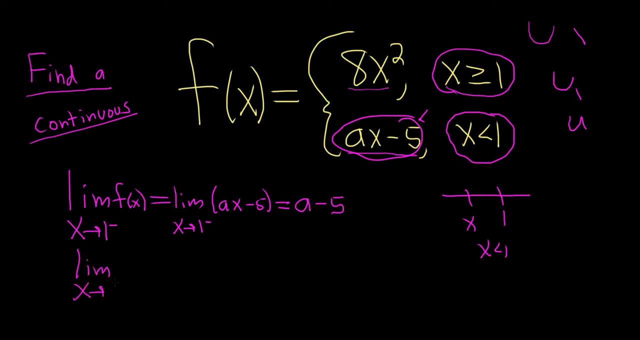 take the limit from the right of f, of x, And so if we're approaching one from the right, that means x is over here. Ah, that means x is bigger than one. That means we use the top piece, right. What a beautiful problem. So this is equal to the limit. Notice, we still. 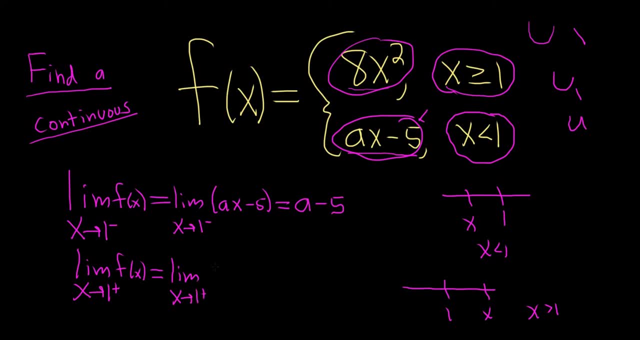 write the limit sign. And now we replace f of x with eight x squared. And again, that's because we're approaching from the right, which means x is over here, And so we're approaching one from the left. Ah, that means x is over here. Ah, that means x is over here. So notice. we caught the turning point and we're approaching it. Let's simulate that again. We plug in the number and it's not in the middle of the world. So we get minus 5 times a mod 5 x squared, which means x is bigger than a plus 3, which means x is bigger than one. So when we give 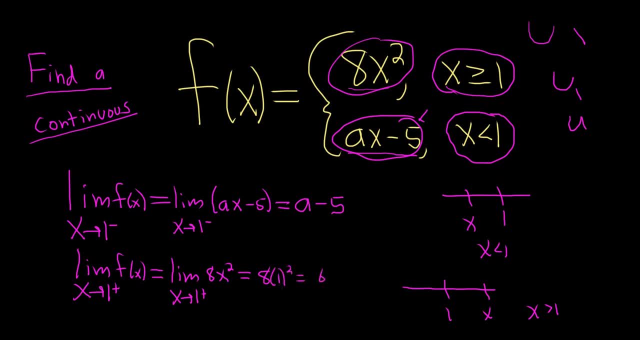 it an 재�ico. we get our limit right, which means x is bigger than a plus 3, right? So we use the top piece. We can evaluate this limit. We plug in the number and drop the limit notation, so we get eight times one squared, which is just eight. So from the 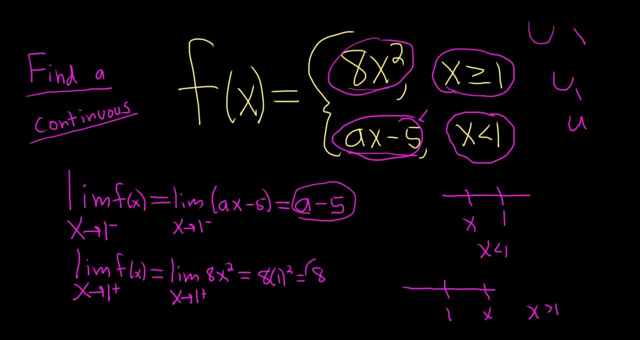 left we get a minus five. From the right we get eight. We want the limit to exist because we want it to be continuous. We're trying to force continuity. So what we do is we set the limits equal to each other. That means that a minus 5 must be equal to 8.. 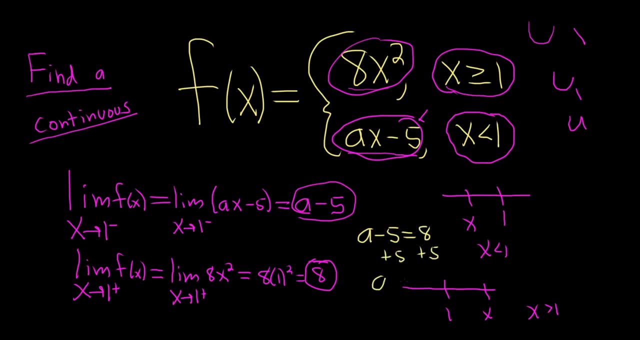 Adding 5 to both sides gives us the wonderful value of 13,, and that is the value of a, which makes this function continuous. I hope this video has been helpful. Good luck.